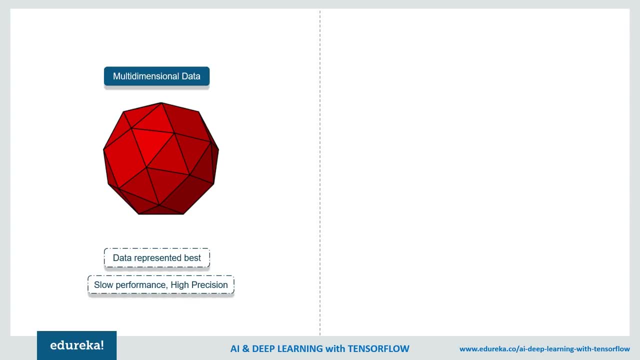 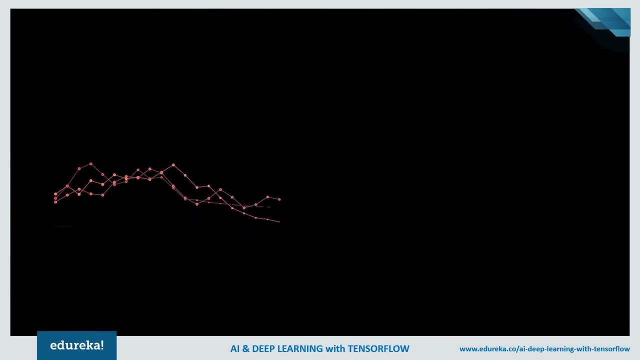 original high dimensional structure, the data represents itself best. sometimes we might need to reduce its dimensionality. The need to reduce dimensionality is often associated with visualizations, but that is not always the case. Sometimes we might value performance over precision. so we could reduce thousand dimensional data to 10 dimensions so that we can manipulate it faster. 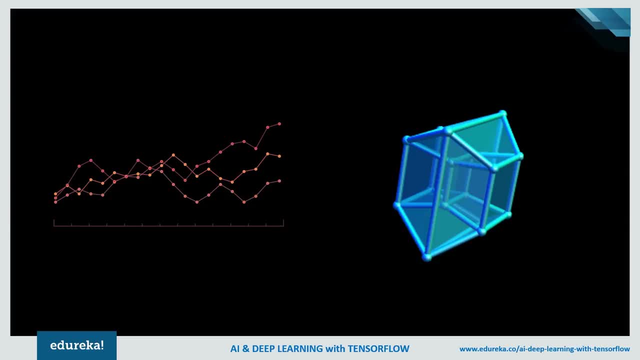 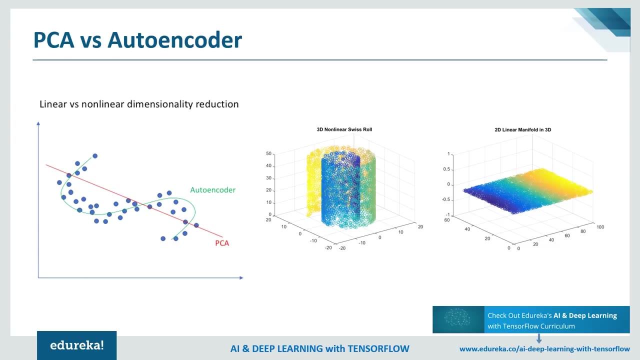 Now the aim of an auto encoder is to learn a compressed, distributed representation for the given data. Now we already have principal component analysis for that, Then why do we need auto encoders? PCA is restricted to a linear map, while auto encoders can have non-linear encoder. 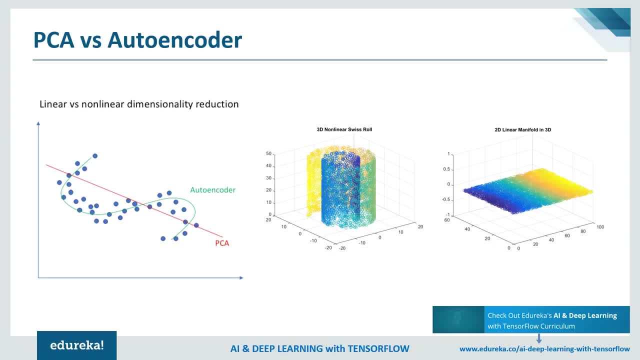 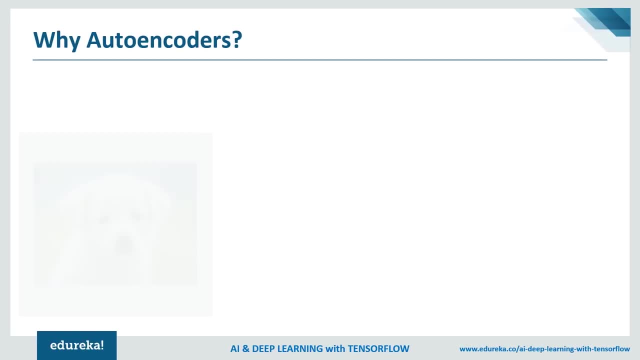 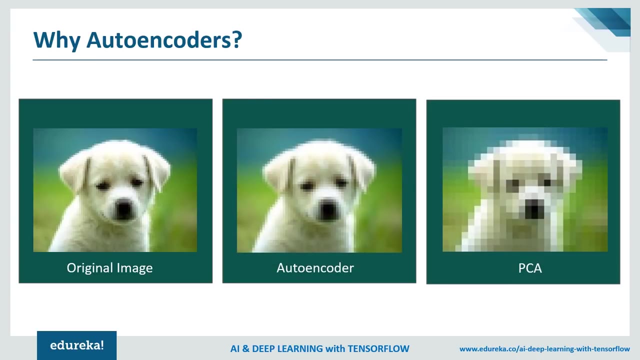 or decoder. Additionally, with an increasing amount of features, PCA will result in slower processing compared to an auto encoder. Now, despite the fact the practical applications of auto encoders were pretty rare some time back, today data denoising and dimensionality reduction for data visualization are considered as two main interesting practical applications of. 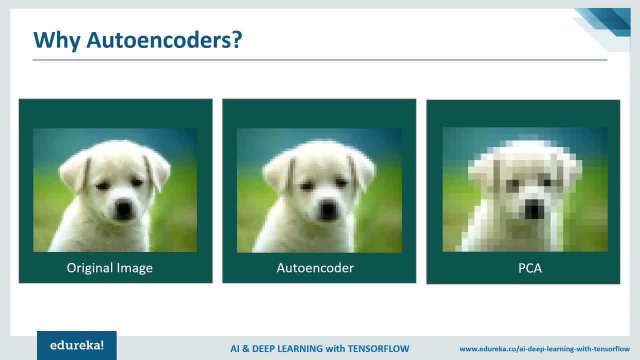 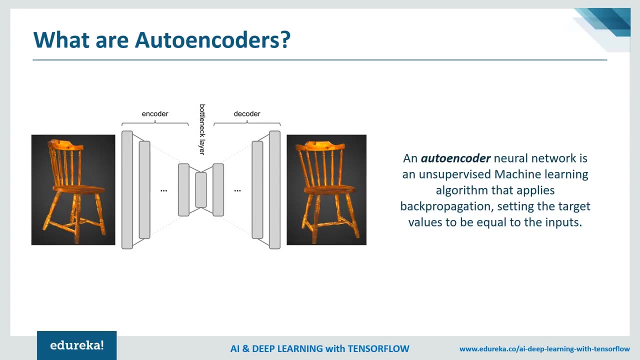 auto encoders. With appropriate dimensionality and sparsity constraints, auto encoders can learn data projections that are more interesting than PCA or other basic techniques. So let's have a detailed look into what are auto encoders. These are simple learning networks that aim to transform 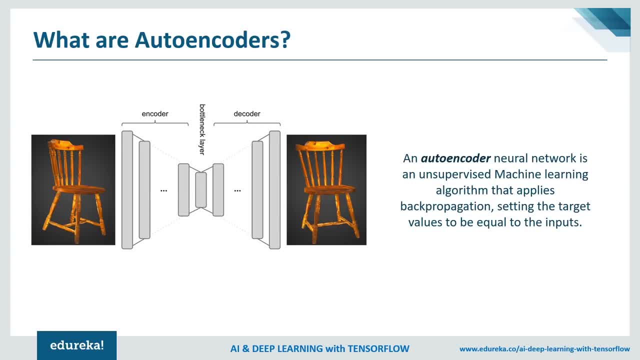 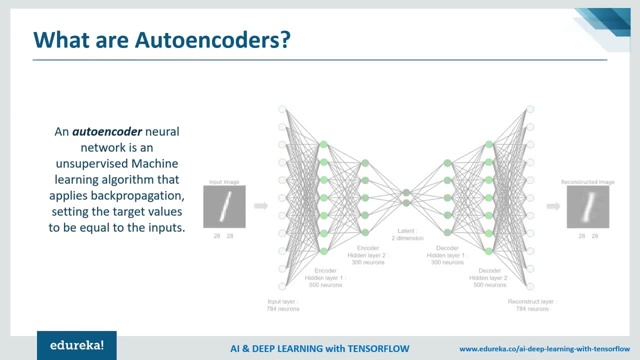 inputs into outputs with the minimum possible error. This means that we want the output to be as close to input as possible. So for that we add a couple of layers in between the input and the output, and the sizes of these layers are smaller than the input layer, Let's say the input vector. 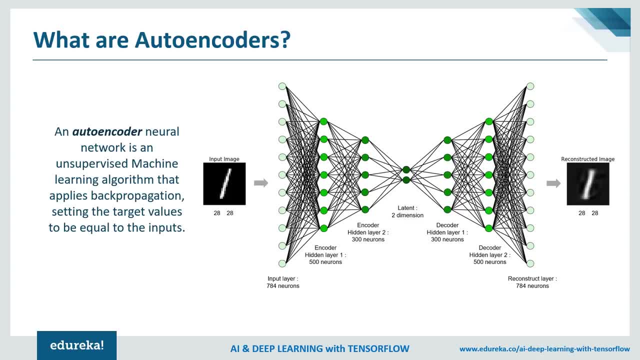 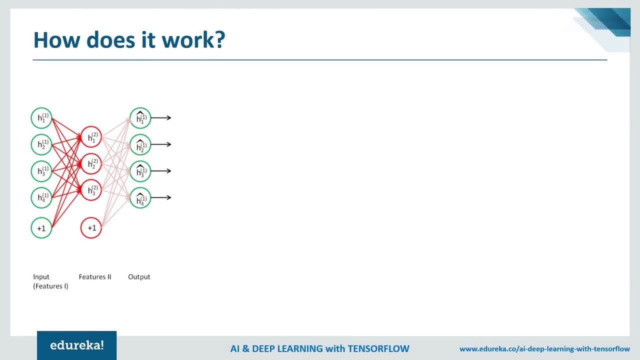 has a dimensionality of n, which means that the output will also have a dimensionality of n. Now we can make the input go through a layer of size p, where the value of p is less than n, and we ask it to reconstruct the input. Now let's see how it actually works. So the main goal of these neural 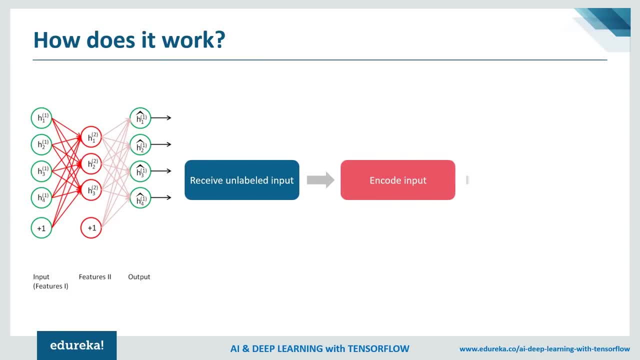 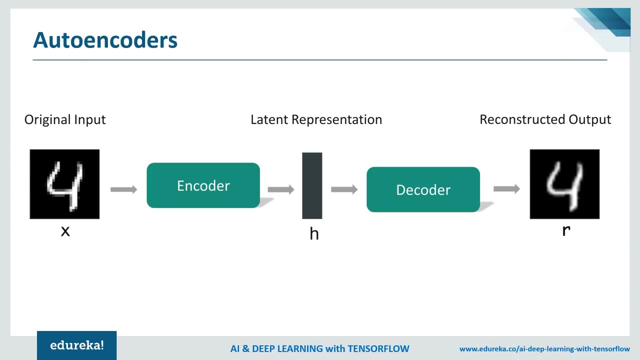 nets is to take unlabeled inputs, encode them and then try to reconstruct them afterwards based on the most valuable features identified in the data. Now, mathematically speaking, an encoder is a model that takes a vector input x and maps it into a hidden representation h using an encoder. Now the 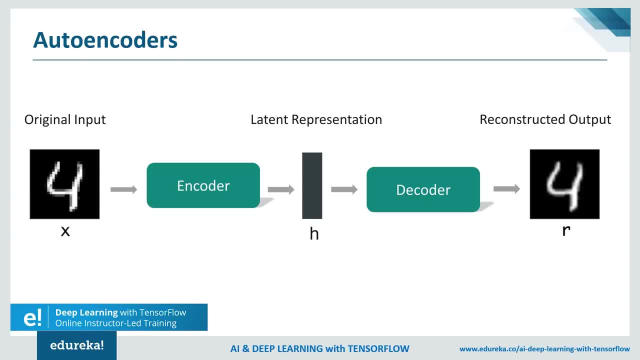 hidden representation h, often called code, is then mapped back into the space of x using a decoder. Now, the goal of the auto encoder is to minimize the reconstruction error which is represented by a distance between the input, x, and the output. The code h typically has less dimensions than x. The encoder compresses the input into a. 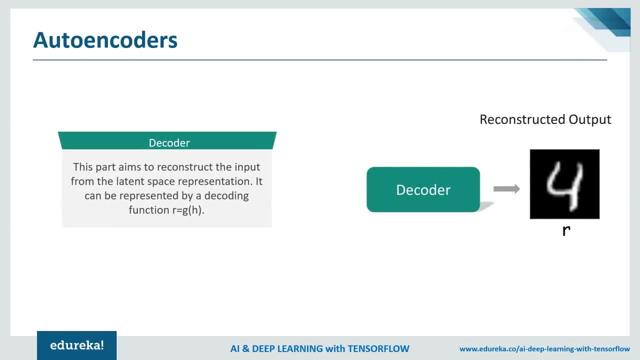 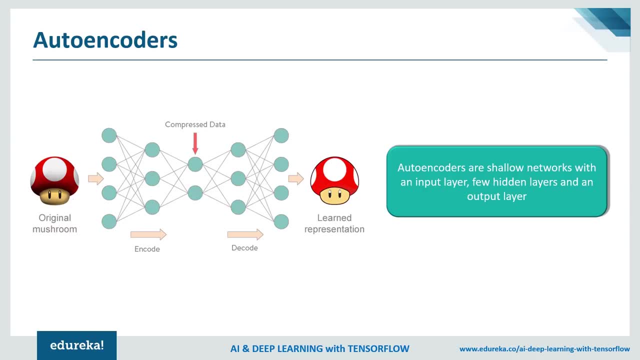 latent space representation and the decoder reconstruct the input from there. Now an idle auto encoder model is sensitive to the inputs to accurately build a reconstruction. Also, it is insensitive enough to the inputs that the model does not simple memorize or overfit the training data. Now the bottleneck is a key attribute of our network design. 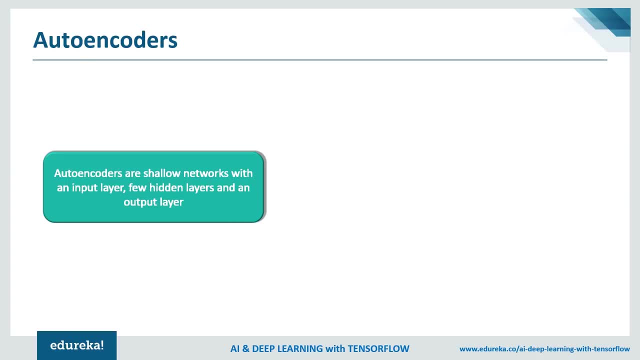 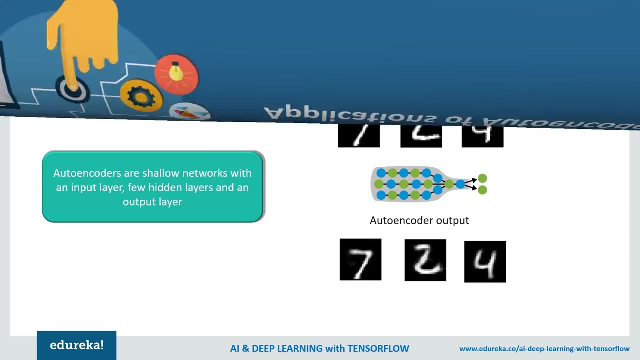 Without the presence of an information bottleneck, our network could easily learn to simply memorize the input values by passing these along the network. Now, a bottleneck constrains the amount of information that can traverse the full network, forcing a learned compression of the input data. So now let's have a look at the applications of auto encoders. So auto encoders are used for? 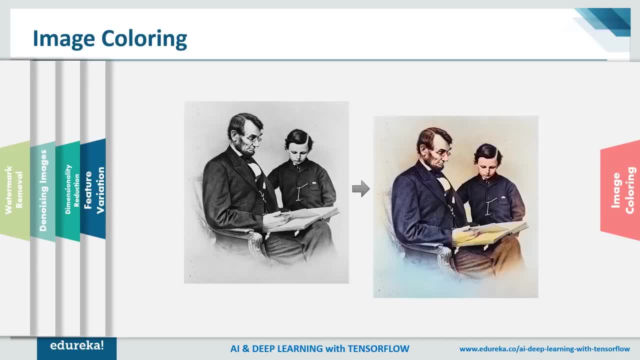 converting any black and white picture into a colored image. Depending on what is in the picture, it is possible to tell what the color should be. For example, the leaves of trees are generally green, the sky is blue and the clouds are white, So all that is needed to be done is to make a computer be able to do this. 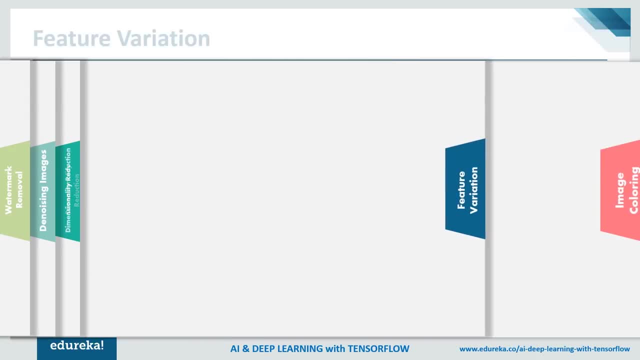 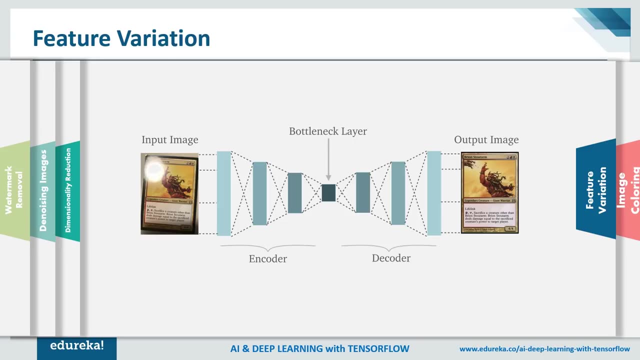 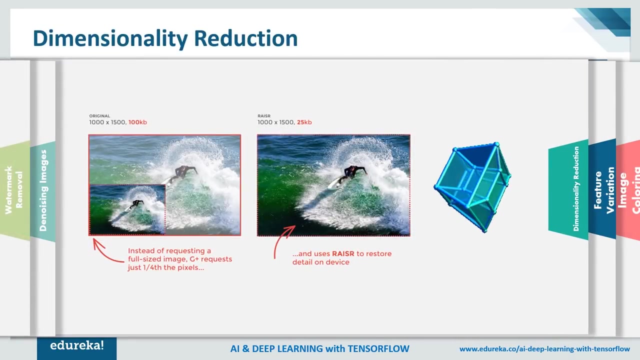 and that is where auto encoders step in. In case of feature variation, it extracts only the required features of an image and generates the output by removing any noise or unnecessary interruption. Using auto encoders, it helps in providing the similar image, along with a reduced dimensional. 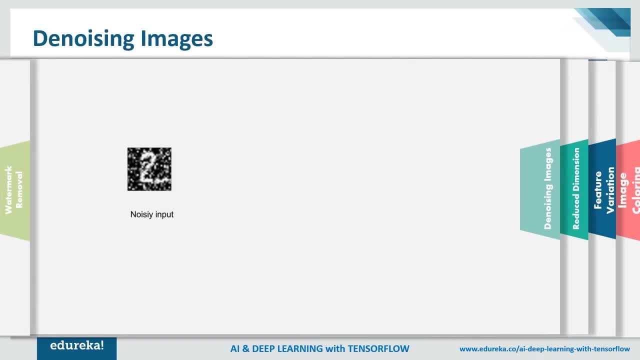 value. Now, during the training, the auto encoder learns to extract important features from input images and ignores the image noises because the labels have no noises. The input seen by the auto encoder is not the raw input, but a stochastically corrupted version, A denoising auto. 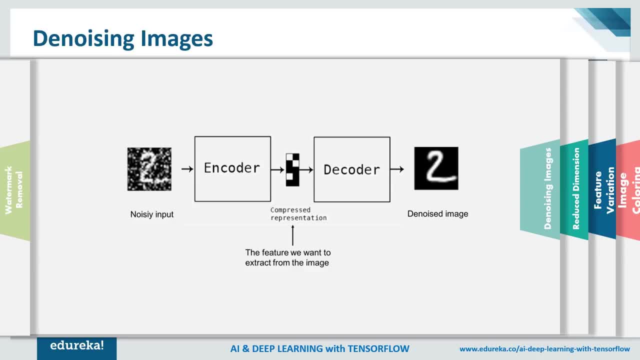 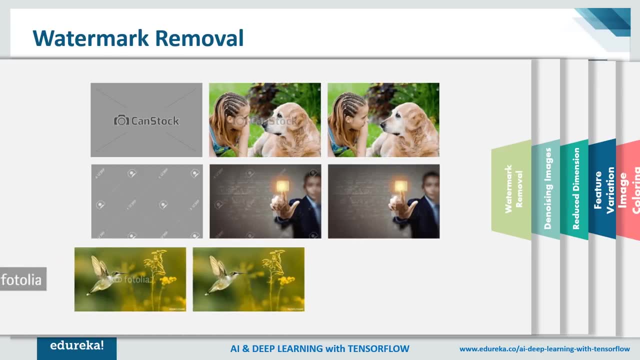 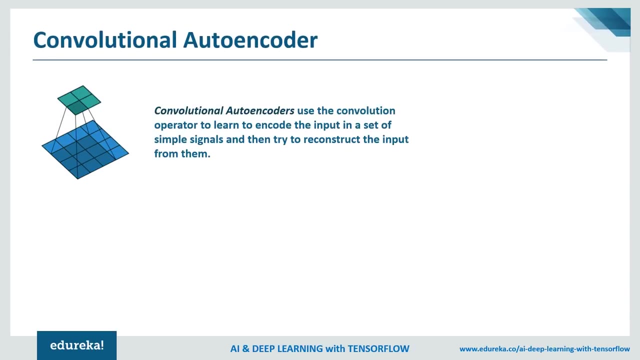 encoder is thus trained to reconstruct the original input from the noisy version. It is also used for audio marks from images or to remove any object while filming a video or a movie. So now let's have a look at the different types of auto encoders. First one is the convolutional. 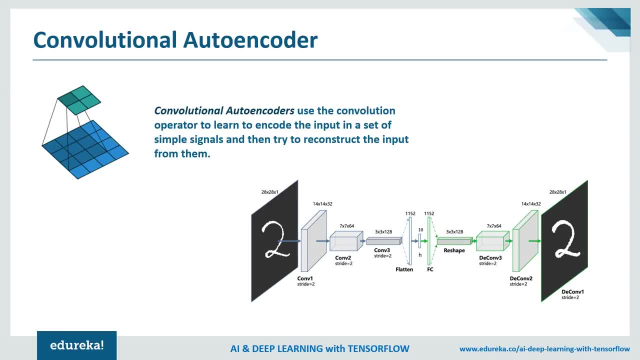 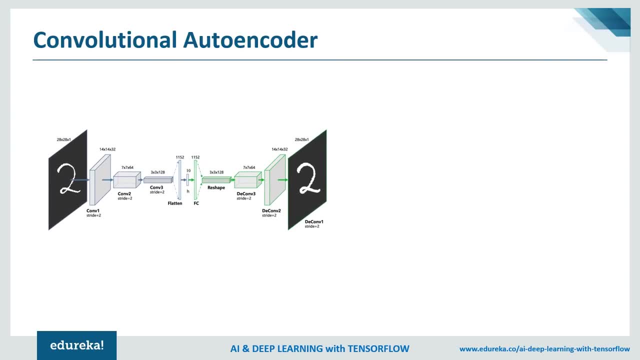 auto encoders. The convolution operator allows filtering an input signal in order to extract some part of its content. Auto encoders, in their traditional formulation, do not take into account the fact that a signal can be seen as a sum of other signals. Convolutional auto encoders use 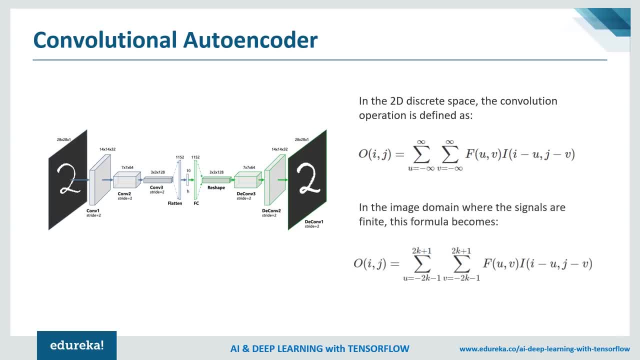 a convolution operator to exploit this observation. These two equations depict the convolutions operations in 2d latence space and image domain, where oij is the input pixel in position ij, f is the convolution filter and i is the input image. Now let's have a look at some of the 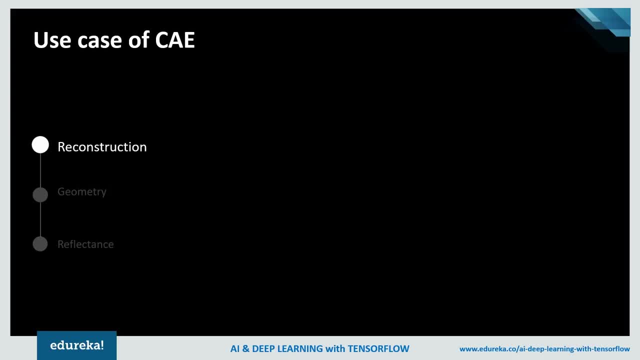 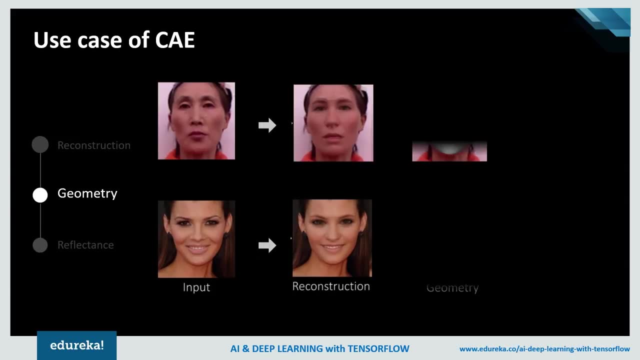 use cases of this auto encoder, So they learn to encode the input in a set of simple signals and then try to reconstruct the input from them. They can also modify the geometry or the reflectance of the image. Next is the variational autoencoders. 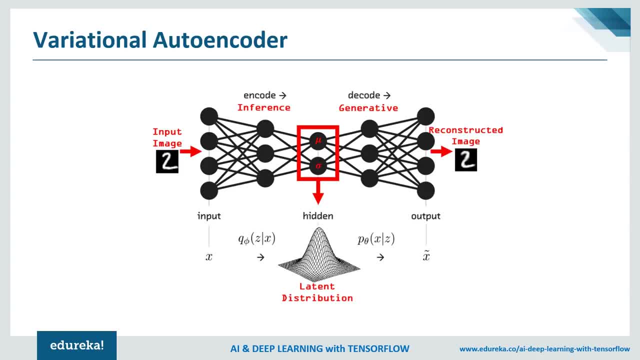 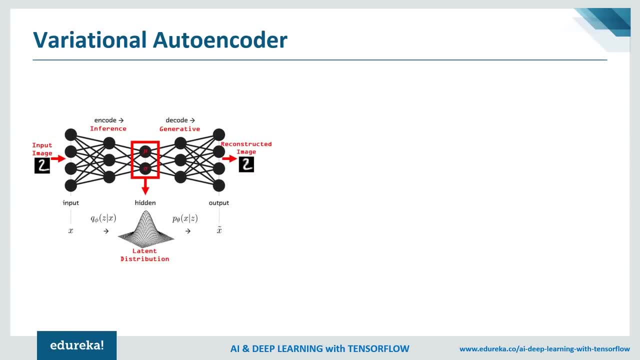 They let us design complex generative models of data and fit them to large data sets. Now they can generate images of fictional celebrity faces and high resolution digital artwork. The encoder is a neural network and its input is a data point, X. Its output is a hidden representation, Z, and it has weights and biases- theta. 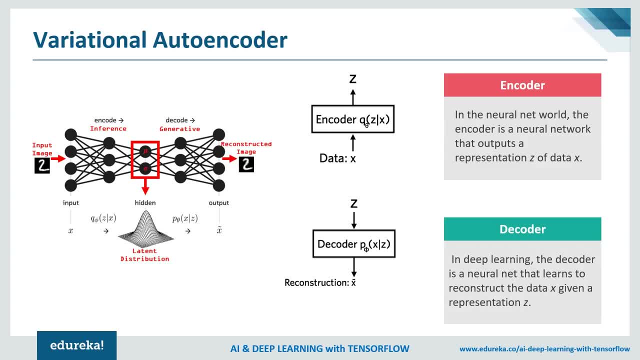 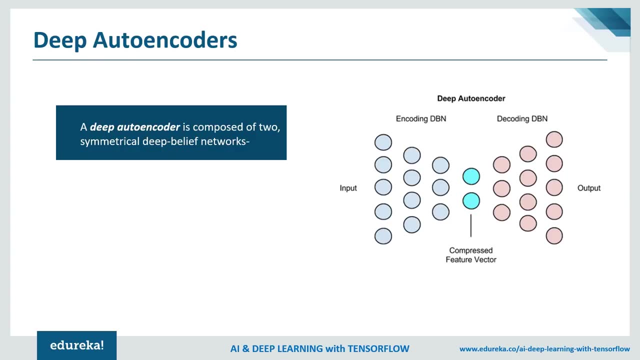 Now the decoder is another neural net. Its input is the representation Z and it outputs the parameters to the probability distribution of the data, and it has weights and biases as phi. Next is the deep autoencoder. It is composed of two symmetrical deep belief networks that typically have four or five. 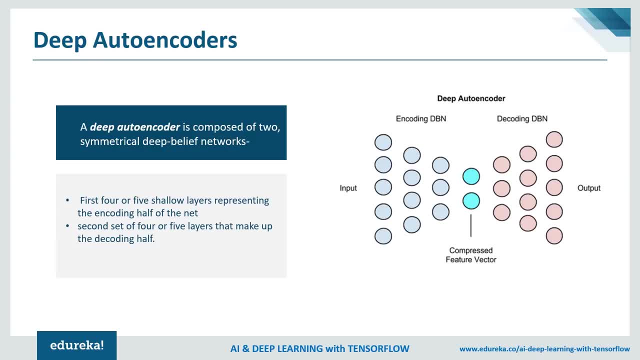 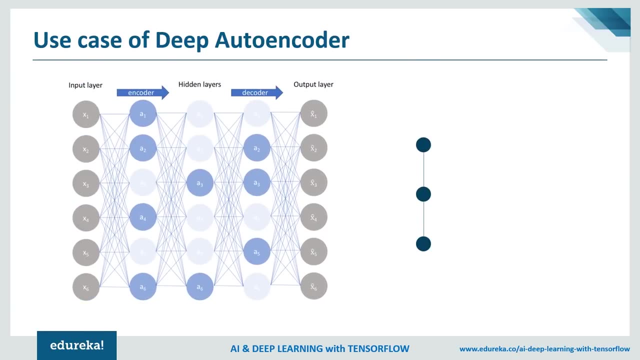 shallow layers representing the encoding half of the net, and second set of four or five layers that make up the decoding half. Now these layers are restricted Boltzmann machines, the building blocks of deep belief networks With several peculiarities. so let's have a look at some of the use cases of deep autoencoders. 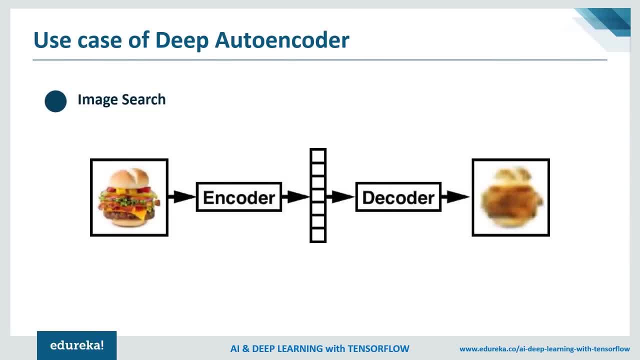 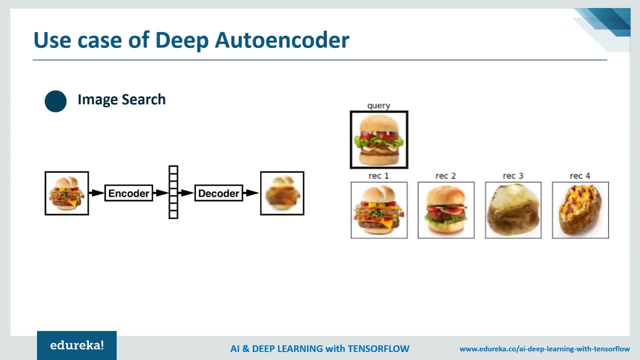 These are capable of compressing images into 30 number vectors. image search therefore becomes a matter of uploading an image, which the search engine will then compress to 30 numbers and compared that vector to all the others in its index. vectors containing similar numbers will be returned for the search query and translated into their matching image. 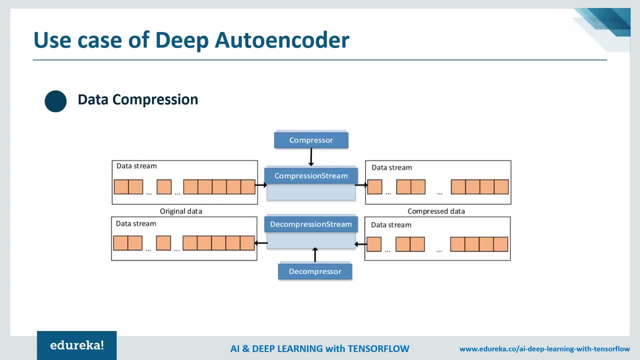 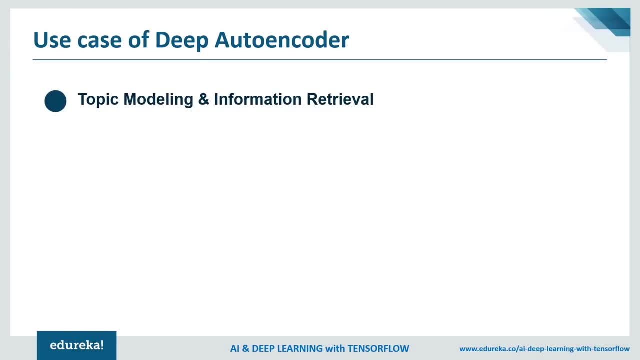 Now, a more general case of image compression is data compression. deep autoencoders are useful for semantic hashing. These are also useful in topic modeling or statistically modeling abstract topics that are distributed across a collection of documents. Now each document in a collection is converted to a bag of words and those word counts are. 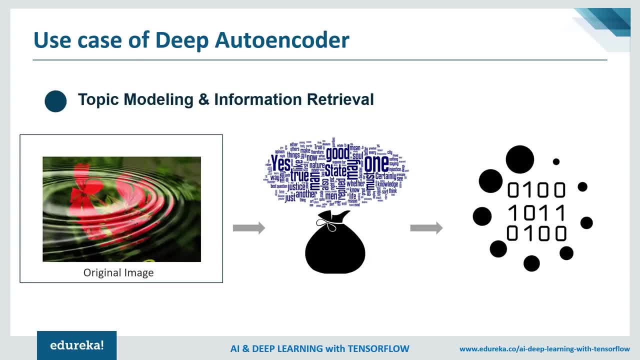 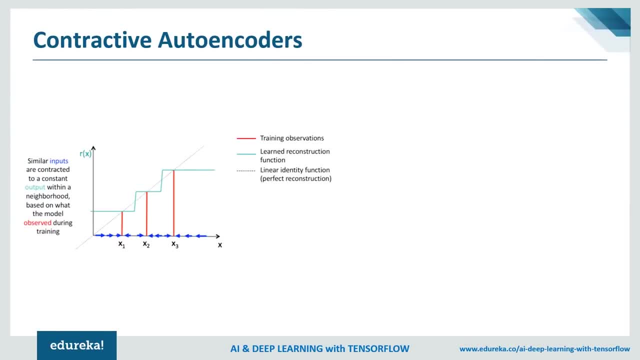 scaled to decimals between 0 and 1, which may be thought of as the probability of a word occurring in the document. The next one Is the contractive autoencoders. These are a type of regularized autoencoders. now, regularized autoencoders also try to learn. 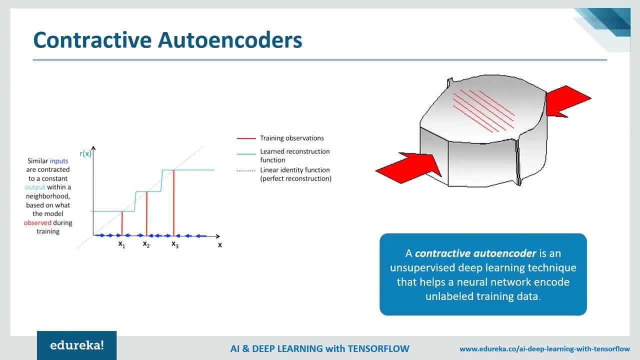 latent variables, but in a different way. rather than limiting the number of latent variables, regularized autoencoders add some sort of penalty or noise to the loss function. Contractive autoencoders are a type of regularized autoencoder and they grow your loss function. 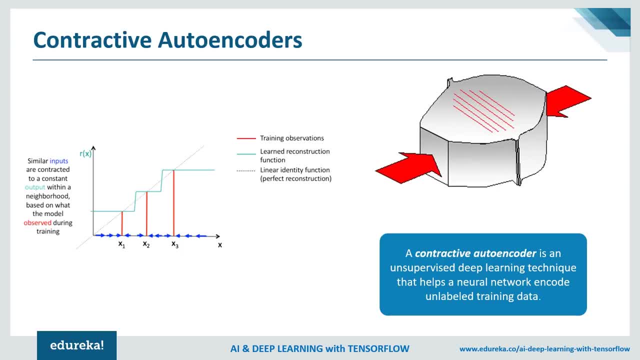 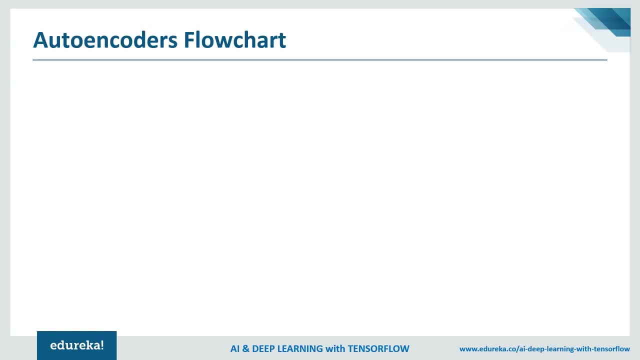 when your derivative is large, encouraging your model to take larger steps to improve gradient descent. Now let's have a look at the flowchart of autoencoders and the steps involved in the process of reconstructing the input. Now it receives the unlabeled images and converts it into sampled patches and then pre processes. 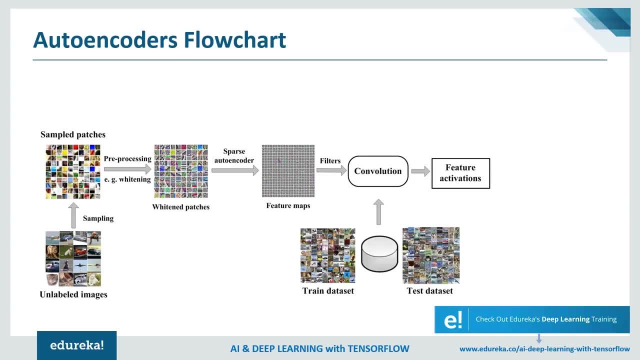 the data. The features are mapped with the train data set for various feature activations, which are then evaluated and pulled into the reconstructed image. Now that we know the various layers involved in autoencoders, So let's have a look at how it actually works. 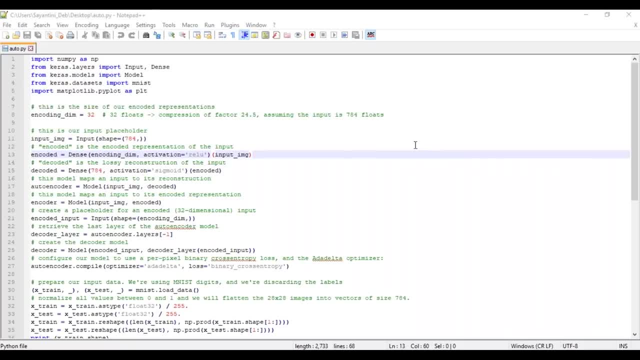 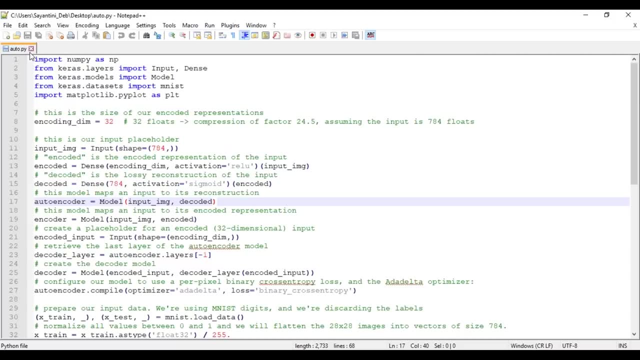 So this is the code for autoencoder that generates a similar output as the input with reduced dimensions. The packages that are needed to be pre installed are NumPy, Keras and matplotlib. So first we define the size of our encoded representations. The encoded representation of the input is declared as encoded, while the lossy reconstruction 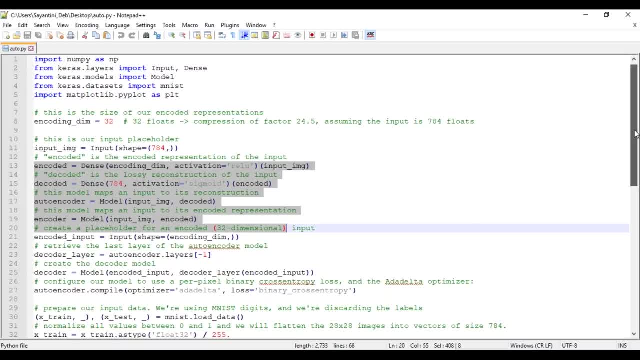 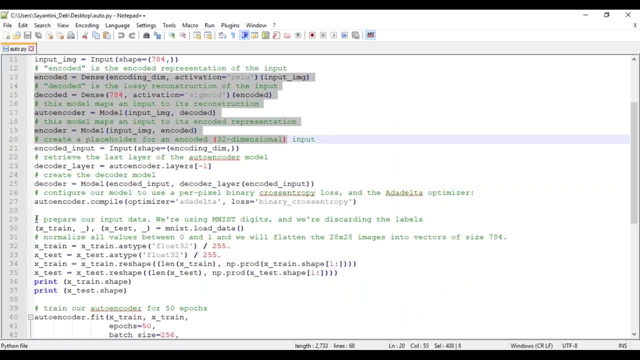 of the input is declared as decoded. The input is then encoded. Now let's have a look at how it actually works. So the decoder is then mapped to its encoded representation in order to create the decoder model. Next, we have to prepare our input data and normalize all the values between 0 and 1..